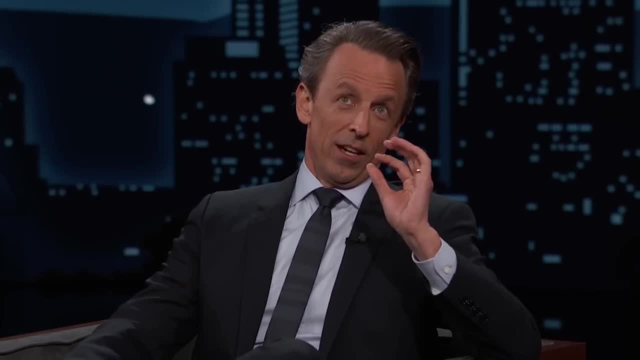 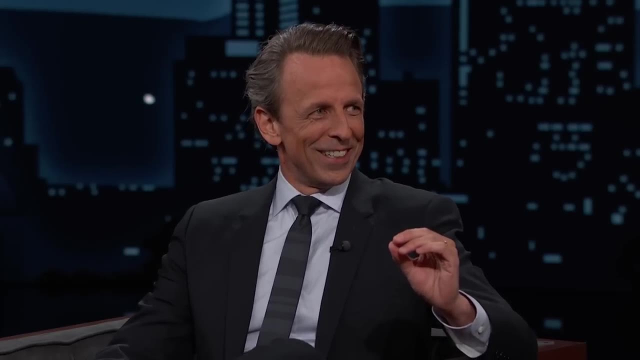 Do you feel like? I always feel like it's unsettling to watch a talk show host as a guest on a different talk show A little bit, Yeah right, It's like seeing your doctor go to another doctor. You're like: why don't you know why you're sick? 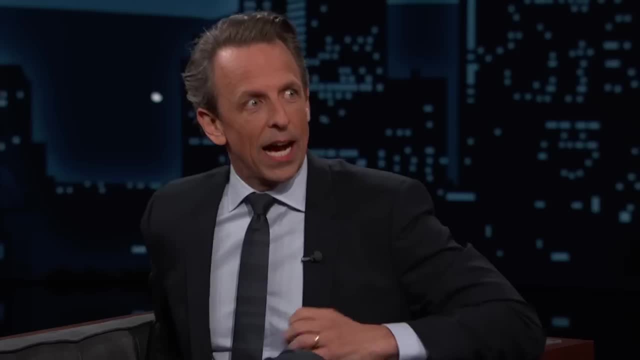 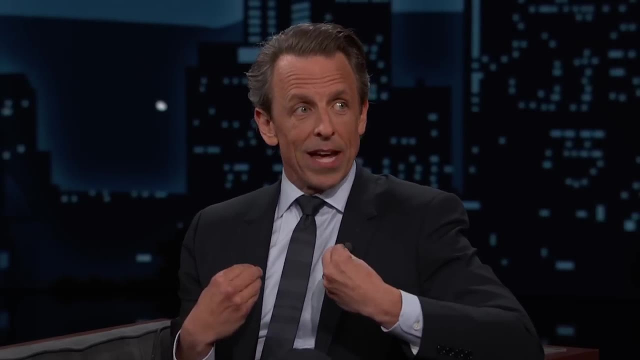 And do you like being the guest, Ana? I don't. I don't either, Because you know, first of all, our lives are made so much fuller by the fascinating guests, The guests that come on our show. But I don't have an interesting life. 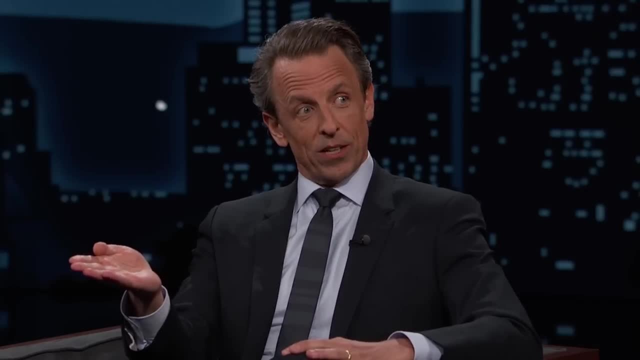 All I have is a life where I hear interesting people tell their stories. So when you are going to say, like, what have you been up to, the best I could be is, like I talked to Jessica Lange last week, You want to hear what she's up to. 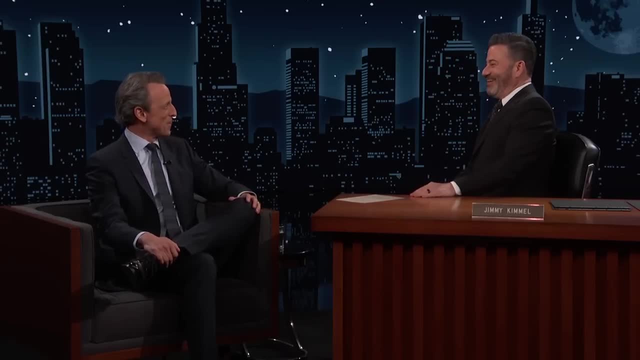 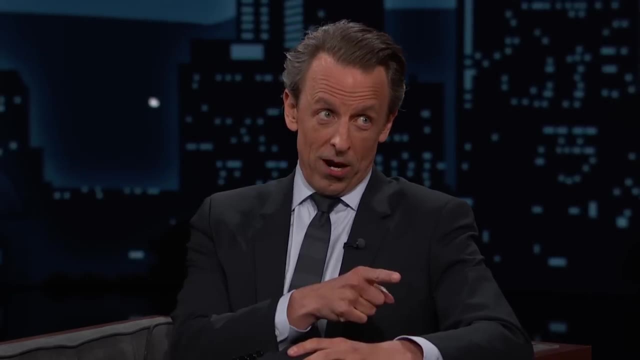 I got. Jessica Lange is living a very full life. What is Jessica up to? She's doing a show on Broadway and it's fantastic. Also, let me tell you the worst part about being a guest on a talk show. You know, Black Puma's been on my show. 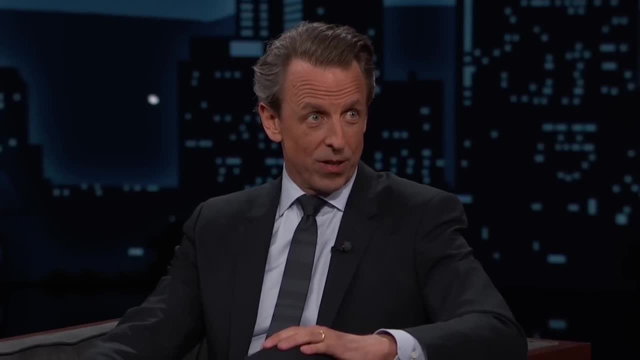 Riley Keough's been on my show Tonight's the first time. I realize we're not exclusive. Oh yeah, I saw Riley. It was very awkward. I'm like, oh so you're doing a lot of these Yeah. 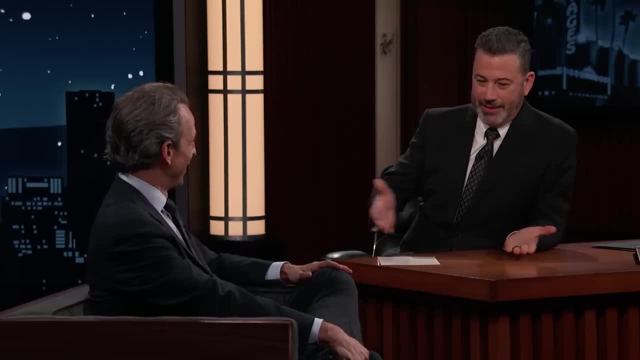 It is funny when you see that, because I'll often see our guests. We have them here on Monday and then two nights later they're over on your show And I thought I was special. Yeah, And I guess we're not. 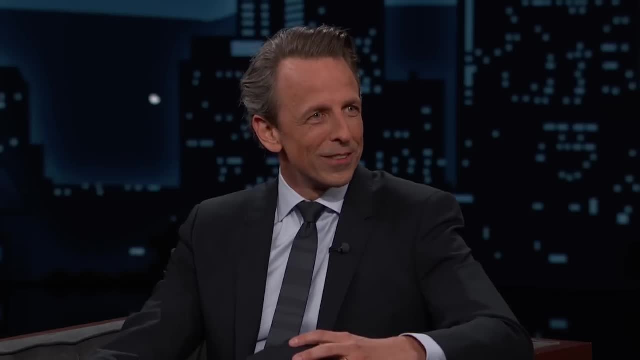 I just feel like there was a thing, and now you're just doing the rounds. Are your kids here on this trip? No, my kids are not here. It's a school week for them, so they're not here, Okay, okay. 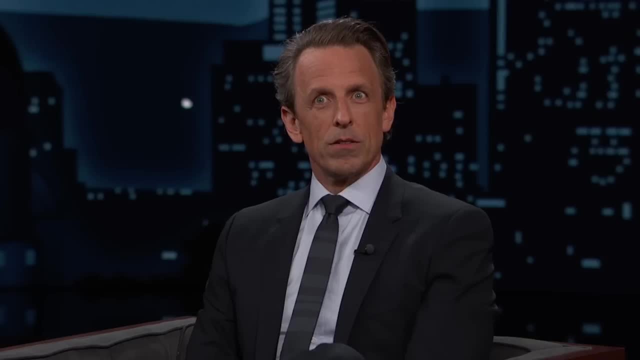 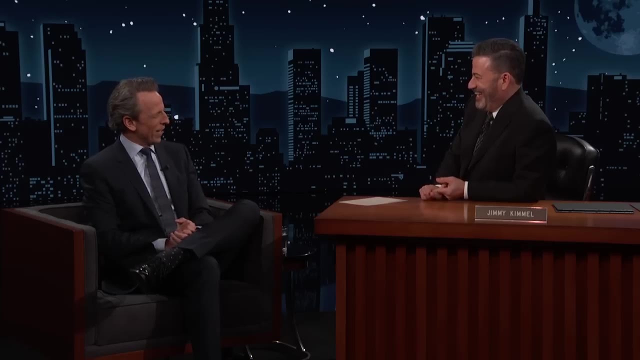 So you don't pull them out. You don't pull them out of the school for silly reasons. Yeah, I think it would be weird to tell their teacher I want them to see me on Kimmel Live, And their teacher would be like: is that not going to be televised? 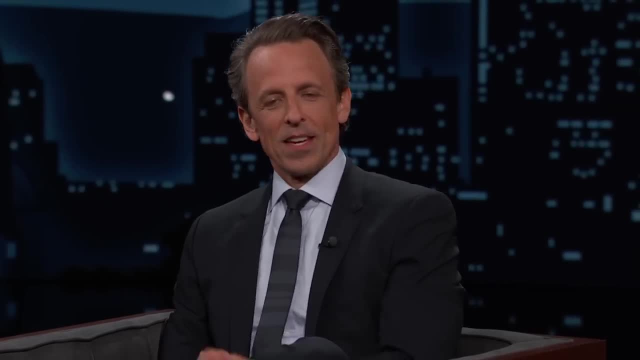 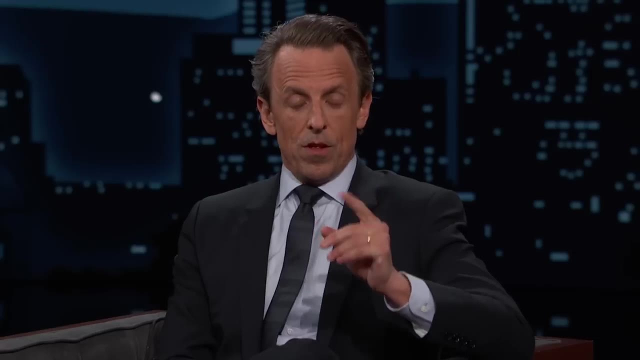 I'm like all right, fair point, fair point. How old are your kids? Eight, six and then the little girl's two and a half, And are they excited about Trump's criminal trial the first day The boys are? 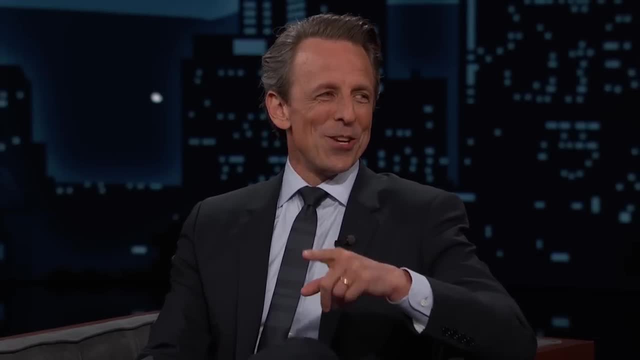 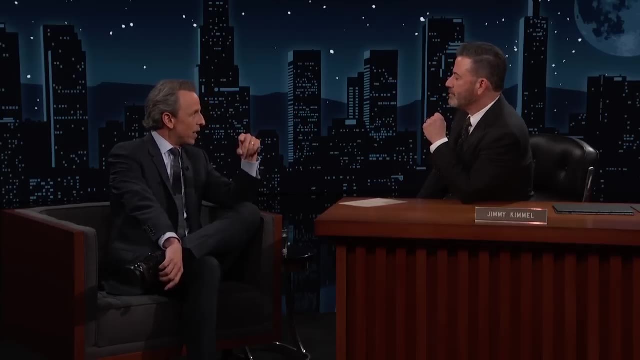 The girl thinks he's being railroaded. She feels as though this is lawfare. She calls it lawfare. By the way, you pulled a fast one on me. What did I do? You invited me to be on this show. This is very exciting for me: first time on the show. 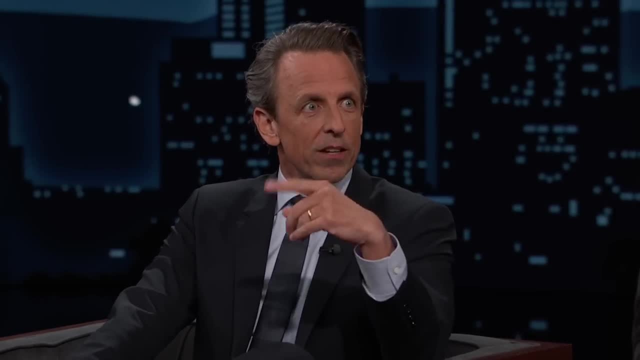 And I cleared. I was like you know what? I'll cancel my shows this week. I realized you got me out here because it's the first day of the criminal trial. That's why I'm dark this week. I know I was wondering about that because this is a terrible night for you. 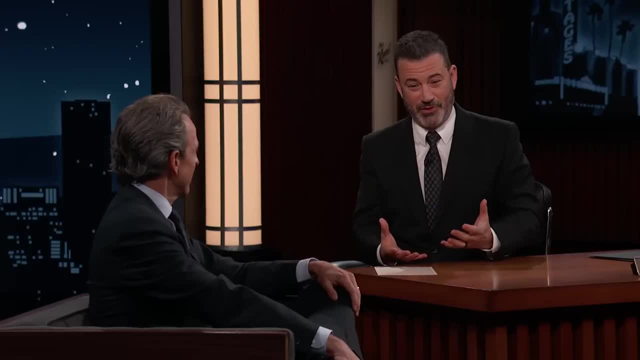 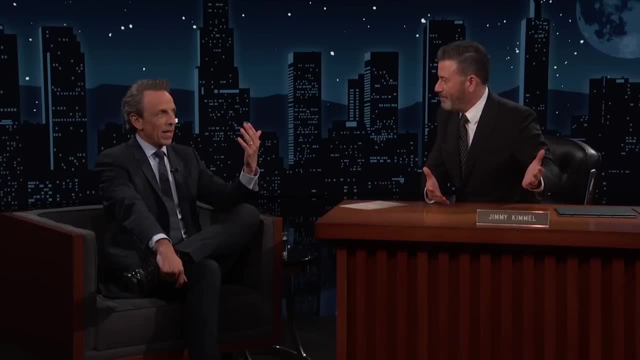 I mean, listen, there's some nights there's a lot going on. There's some nights there's not much going on. This is a night that you think about all weekend. Yeah, I mean, just the clip of Trump in the uphill, clip alone is something that you look forward to. 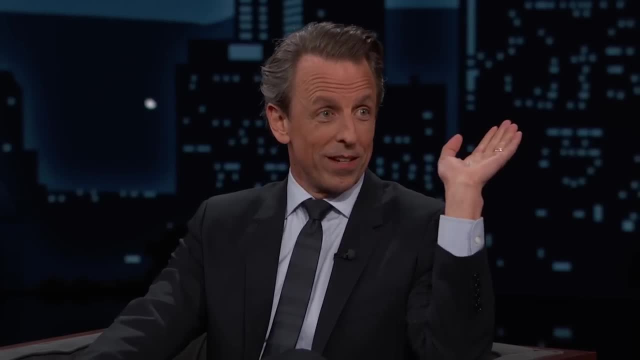 The uphill clip And, by the way there was, There was a good one on Saturday that just got bumped into the trash because of the uphill clip, And then he falls asleep. And then he falls asleep, which is the kind of thing we love. 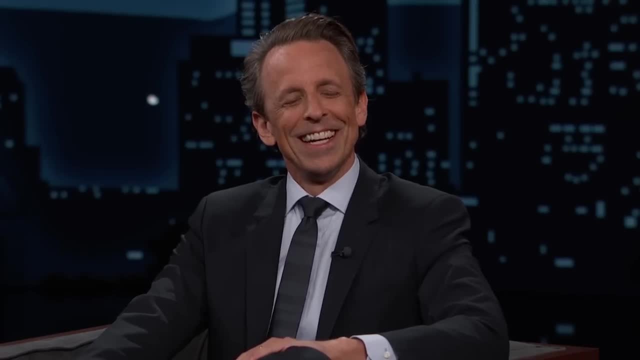 The good news is Jimmy. I think he's going to fall asleep again. He's got a lot of trials and I don't think he's going to get more energy and I think he's going to fall asleep a lot. He's up all night tweeting. 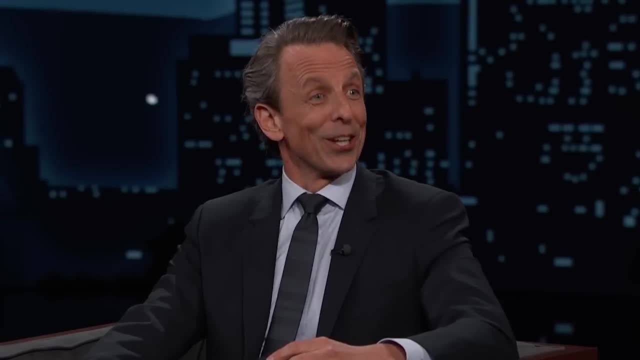 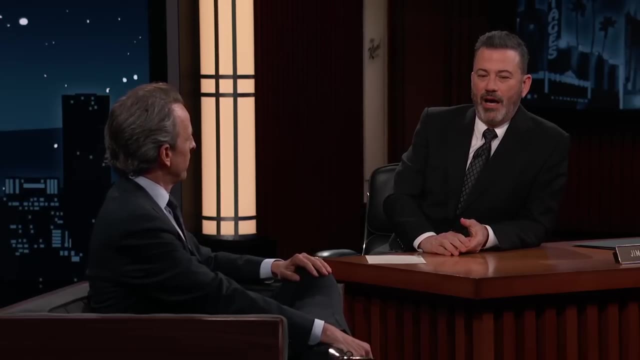 He's up all night. I feel like no one. You know what. I don't think he's getting good advice. I'm sorry, I mentioned your kids and then we got back to Donald Trump. Yeah, Donald, Donald Trump is the father of your children, huh. 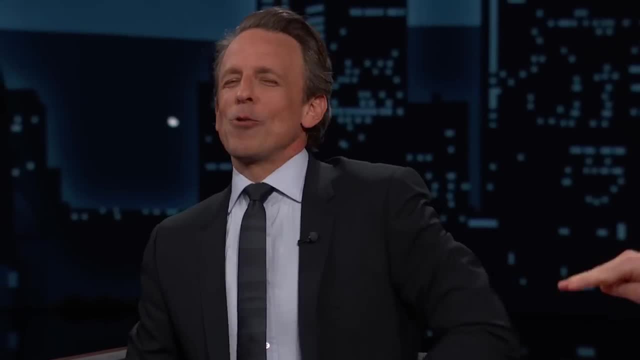 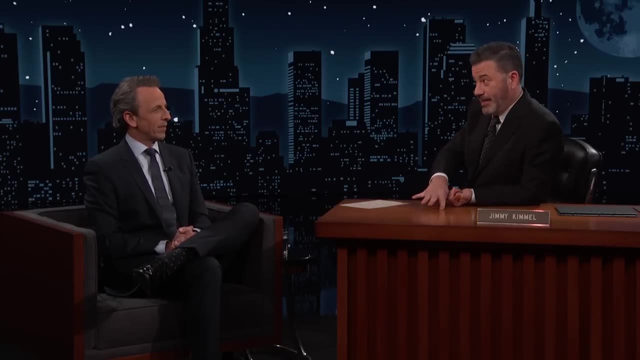 On one of them, but we don't know which one. My wife- it's very coy when I ask her which one. Two boys and a girl? Yeah, Not unlike how he started out with Don Jr, Eric and Ivanka, Yeah. 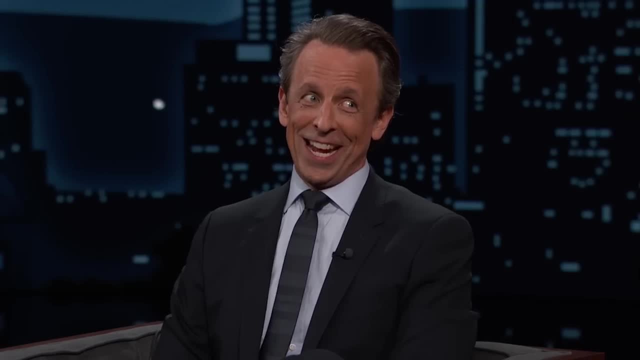 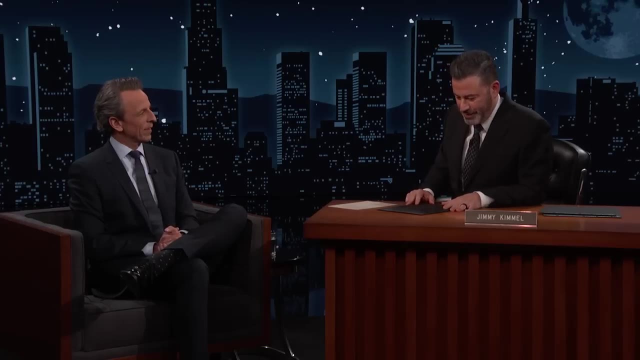 A lot of parallels here. That means I got two more coming with two different ladies. You, I know you. I want to ask you about a photograph that you brought along. This is: you went to the Knicks game with your boy. I brought, so I brought my six-year-old. 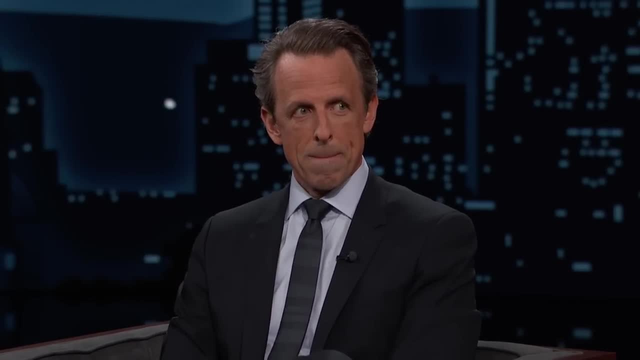 To the first live sporting event of his life. I took him to the Knicks game yesterday. Did he ask you to take him to the game? I was going to take one kid to the Rangers and one kid to the Knicks and I let the eight-year-old choose and he chose Rangers. so the six-year-old got Knicks. 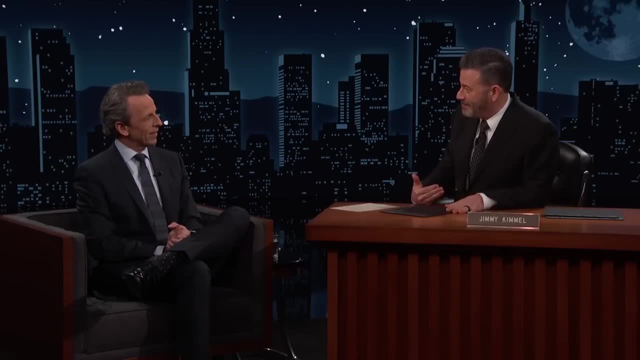 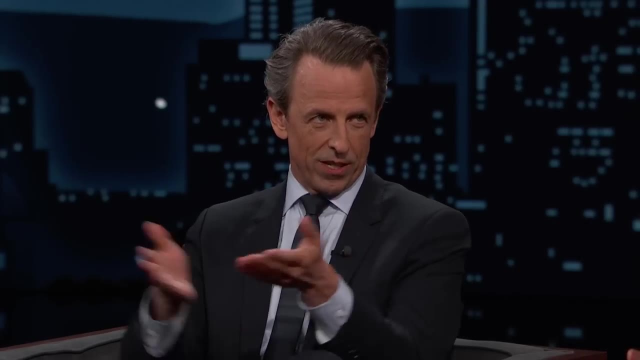 Okay, I recently brought my six-year-old son to a Lakers game and it was a lot of fun. Basketball's the better choice. Hockey's great to watch, but there's no nonsense in between when they take timeouts, because you can't have nonsense on ice. 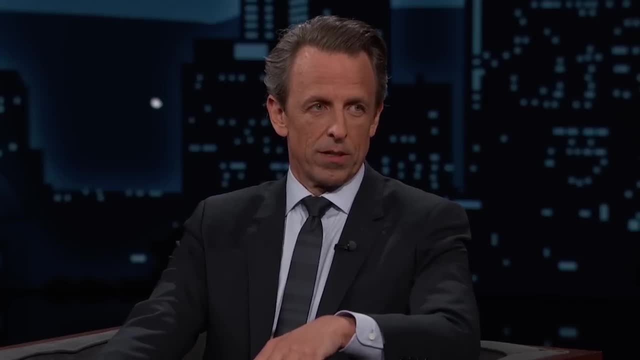 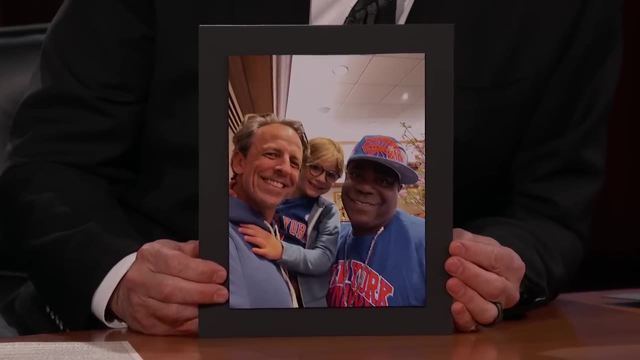 Right, But there's so much nonsense for kids to enjoy at basketball games, And including the presence of one, Tracy Morgan. My son met Tracy Morgan, you guys, Who's always got a lot of nonsense going on. It was, first of all, the highlight of the entire Knicks game was my son meeting Tracy Morgan. 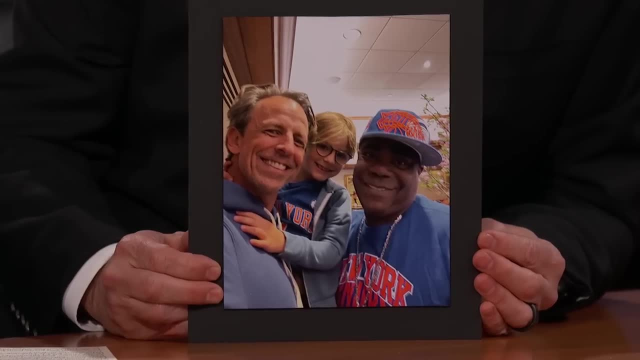 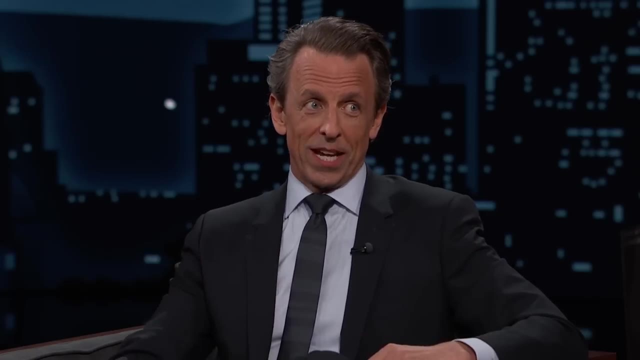 Yeah, Now my son looks very happy. then My son did sort of have a moment of stranger danger with Tracy, because Tracy saw me and walked over and I don't want to get the quote wrong, but it was some version of him saying: ah. 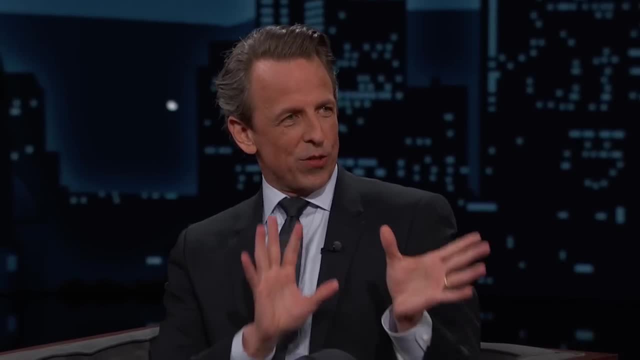 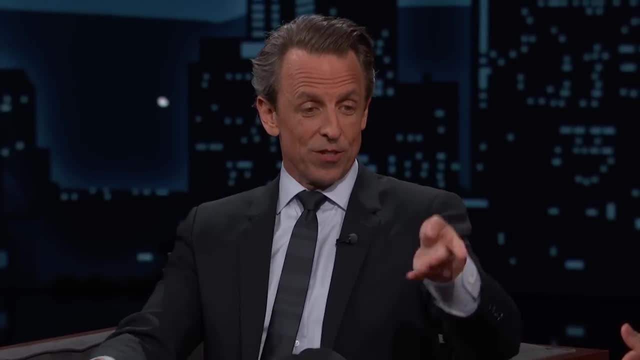 And you know I'm happy that. my son was like: why are you so warm about this? And he talked to him a lot. I was very happy that it was Axel's first game, But then you can see Tracy's wearing all Knicks stuff. 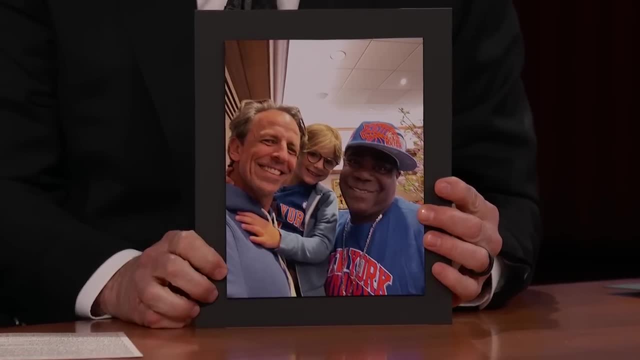 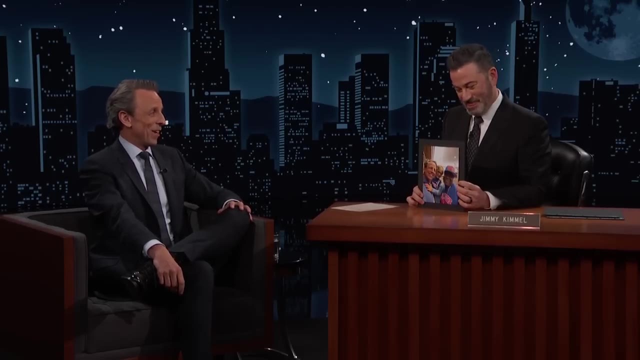 Yeah, Tracy is decked out. Tracy walked away and my son goes. is he one of the playos? And I said he's not, but basketball would be so much better if he was, If you got to have four basketball players and one, Tracy Morgan, on the court at all times. 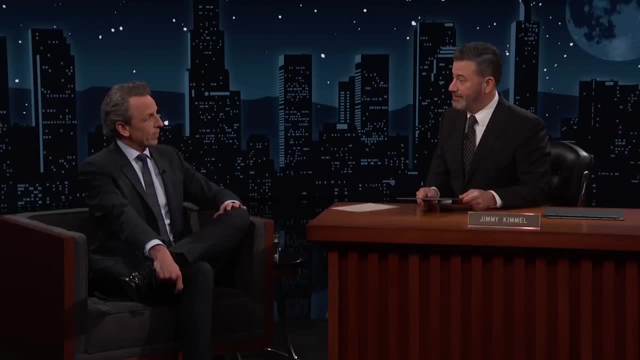 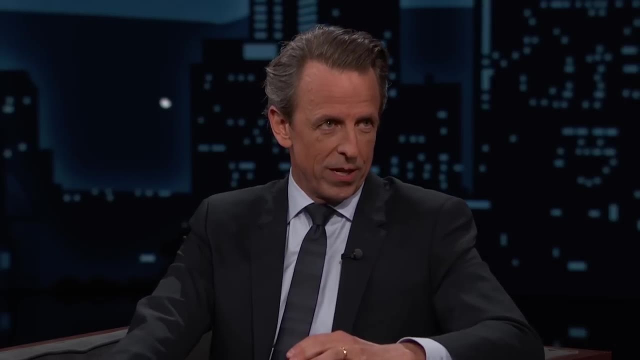 it would be absolutely fantastic. Yeah, I think Tracy would be quite thrilled to be confused with one of the players, for sure. Oh, happily, Even if Tracy was just in warm-ups on the bench, you never even had to put him in. 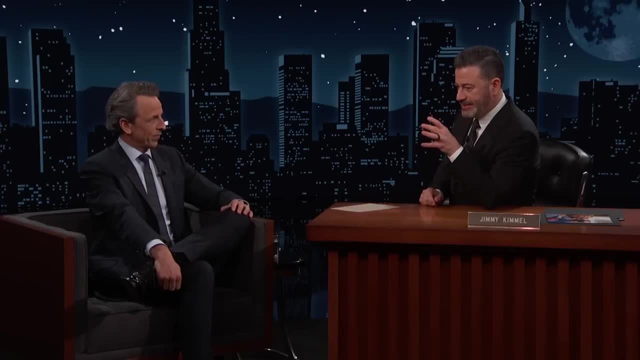 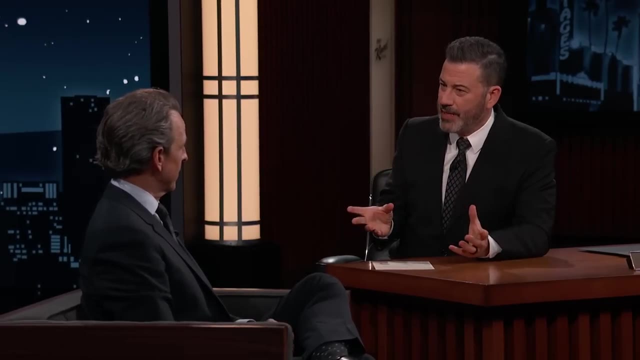 I think he would make the game better. When I took my son Billy to the game, he badly wanted to be on the Jumbotron. Sure, You know, and the kids are very, really eager to be on. I feel like when I was that age I would be hiding from the Jumbotron. 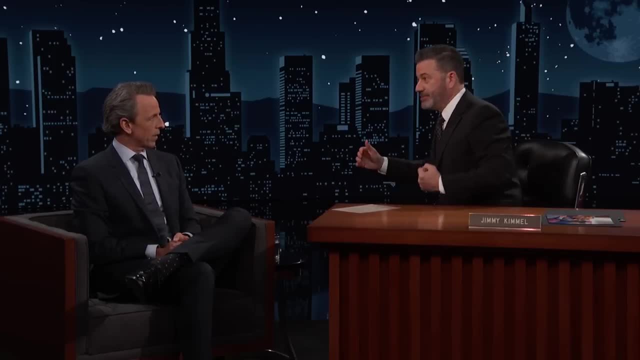 Yes, I think I was very insecure as well, But these children are like they're dancing and they're doing things that you've never seen them do And you know what. At least those kids are working for it, You know. let's be honest. 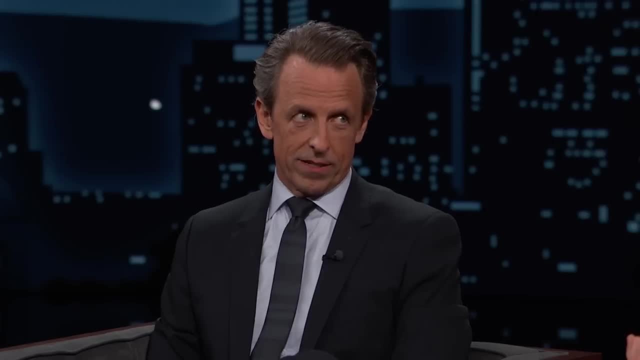 We have children of celebrities. They're going to put them on the Jumbotron. My kid just got a free shot. Oh, your kid got on the Jumbotron. He got on the Jumbotron Because they asked me: like, can we put you on the Jumbotron? 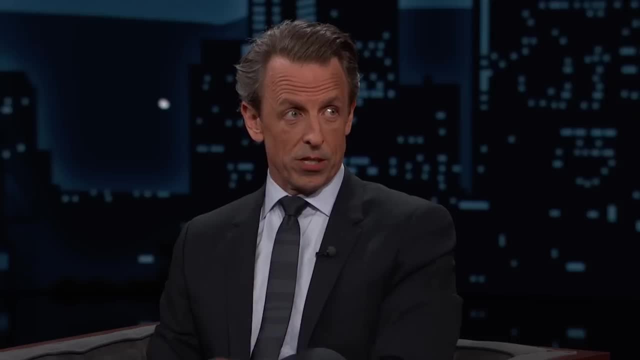 And I said sure, And they said are you okay if your son's on? And before I could even answer he was like yes, And so then they cut to me and him. And you know the players, they were very nice. 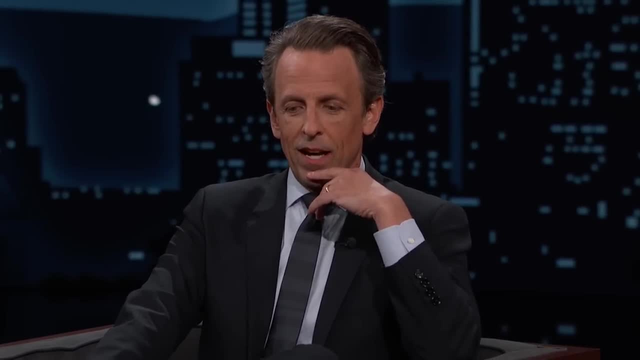 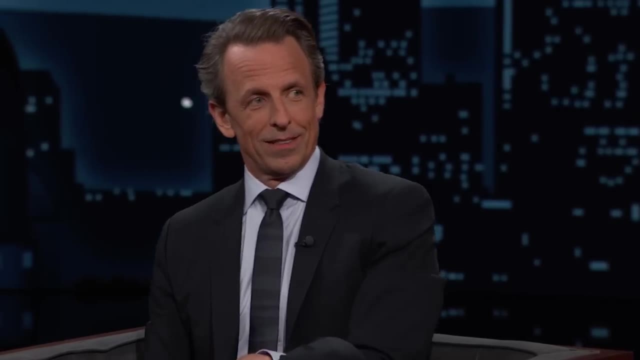 You know, warm round of applause. And then later there was an actress sitting next to us, one seat over, And then, when they cut to her, my son leaned into her shot- Oh really. And I was saying you've got to stop doing that. 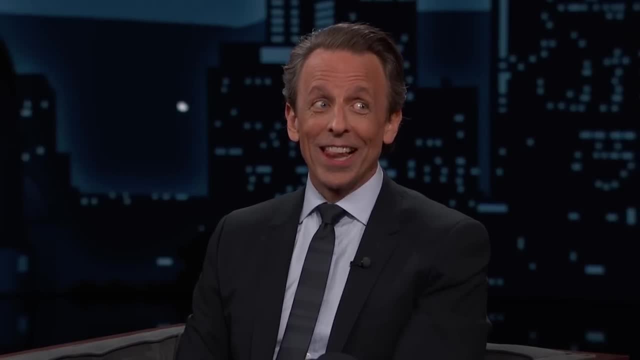 And he's like: they love me. I don't know if you're here, They love me. Would this actress happen to have been Jessica Lange? It wasn't Jessica Lange, I'm sorry. No, because I hear she's got a show on Broadway. 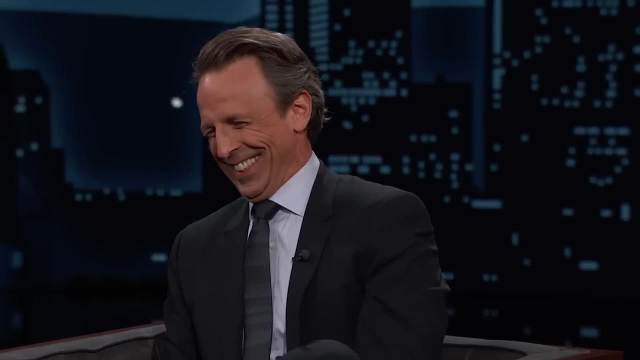 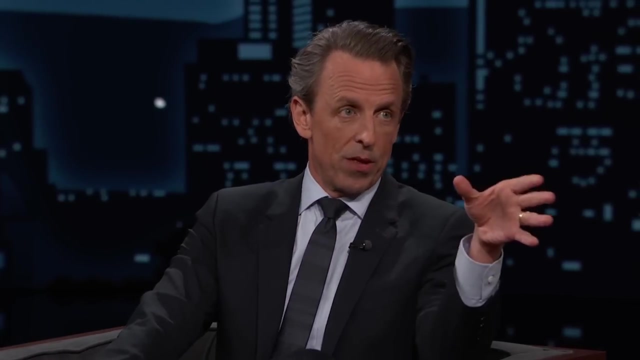 You know what. We've talked enough about Jessica Lange. But I brought my eight-year-old to the Rangers game. Same question. They asked me: do you want to have your son on, Are you okay with it? And he said absolutely not. 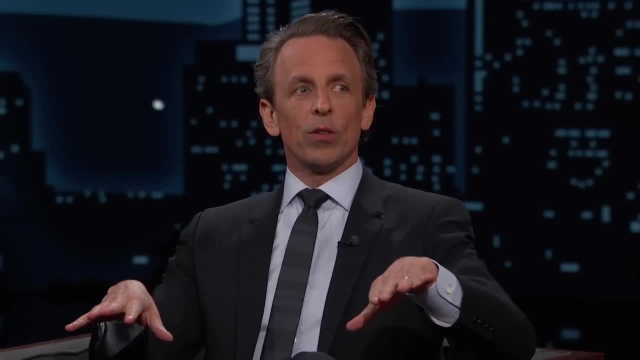 Oh, he didn't want to be on. My eight-year-old did not want it at all And he was nervous the whole time until they put me on that they were going to catch him off guard. He did not want to be on screen. 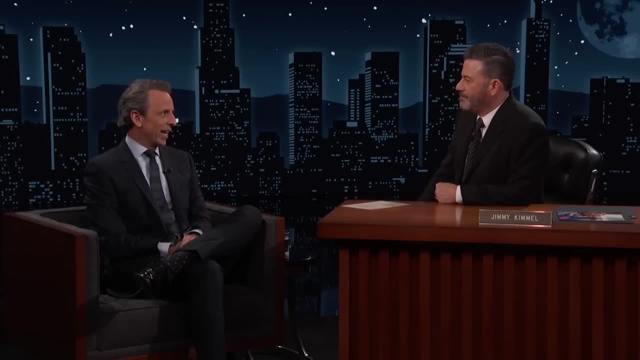 And then he could relax. Yeah, Because, yeah, he's drinking beer. He didn't want to see that. Yeah, he's like. this is everything we're doing here. Dad is against the law. We should not be on camera. 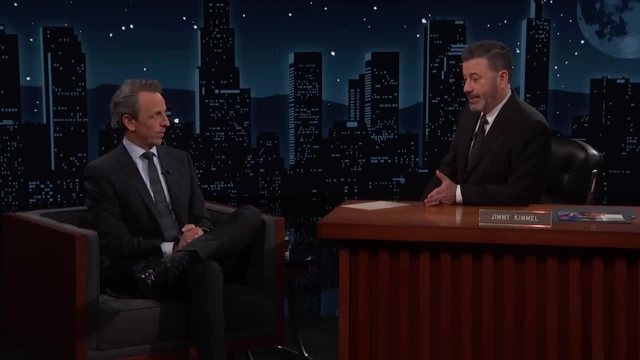 I need to bring something up to you. I don't know if you're aware of this. It's something I probably should have addressed privately. Yeah, Your brother, Josh Myers. Yeah, Younger brother, Uh-huh, Very funny. 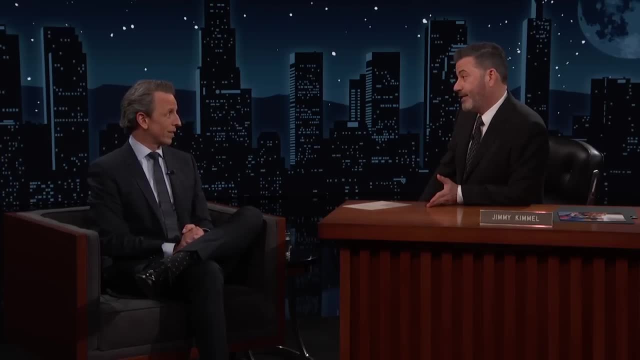 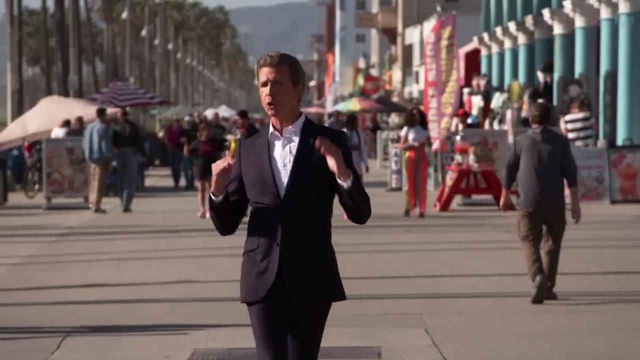 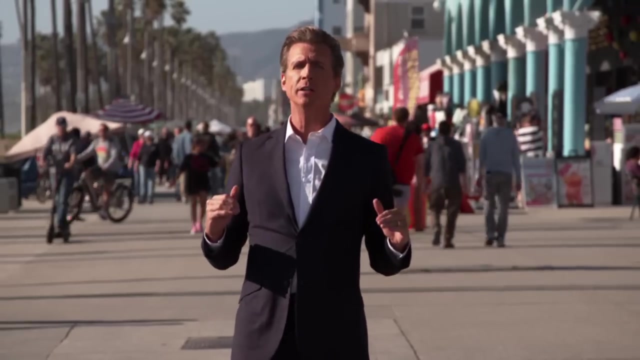 Very loyal to me, Has been making regular appearances on our show as California Governor, Gavin Newsom. I believe we have a clip- Yo yo, It's your number one, bro GovGav, Giving you the 411 about a proposition that's not only important, but is also hella rad. 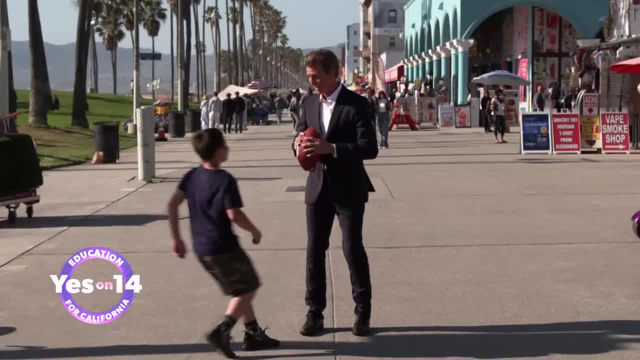 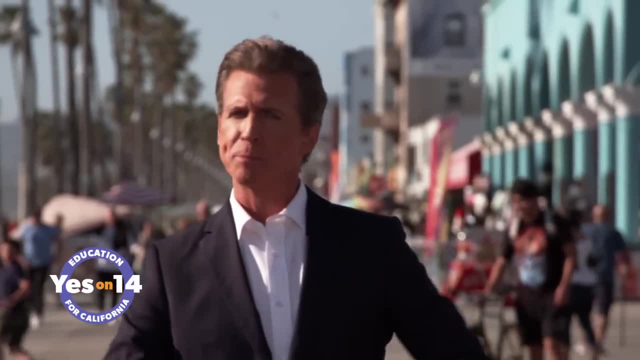 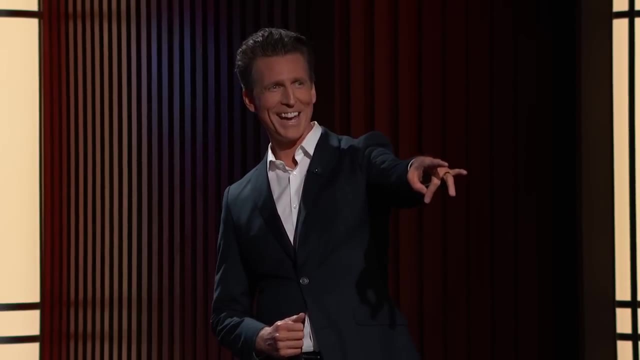 Proposition 14 for education. Hey, go long. There's nothing more imperative than educating our tiny dudes, little ladies, than all the other ones. It's remarkable. Oh, there he is. Oh, Right on, Right on. Well, we have a special visitor with us tonight. 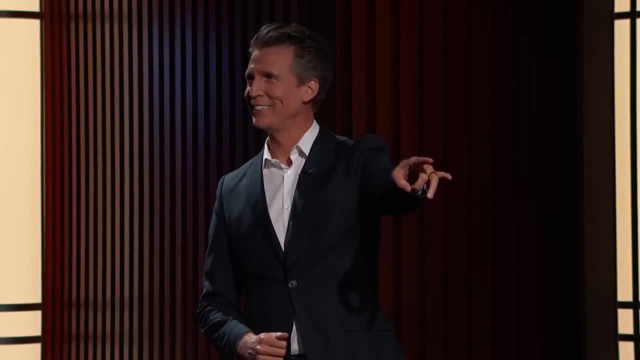 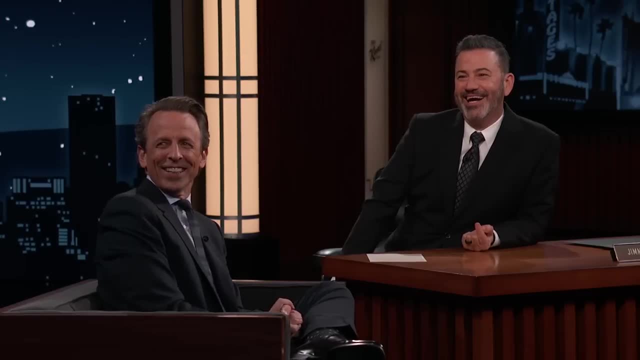 From California. Gavin Newsom is here tonight. Oh yeah, Yes, Yes. What's up, Jimmy? What's up Suf? What? Why are you still in character? Oh man, You wouldn't believe what you get away with when people think you're the governor. 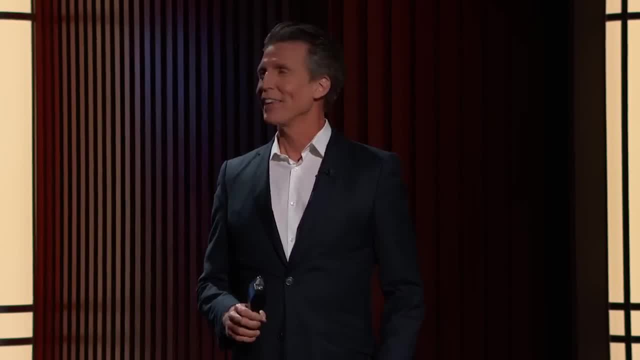 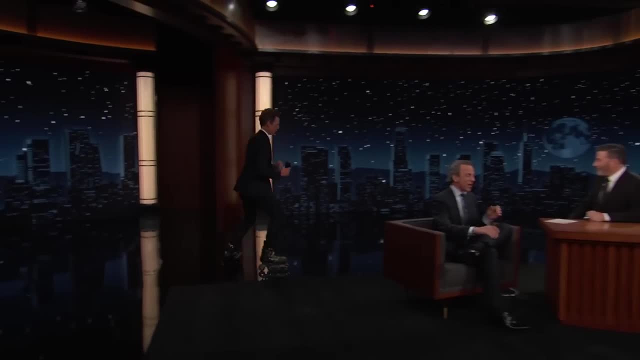 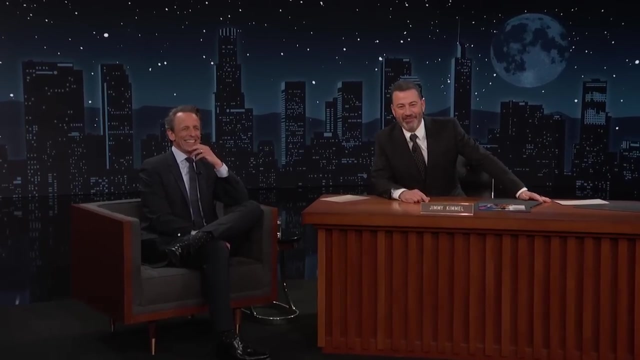 Some cop just gave me a taser. Now, if you'll excuse me, I'm going to go legalize cocaine. Oh, he's on a plate. Wow, Oh my gosh. That's Josh Myers. More with Josh's brother Seth, after this. 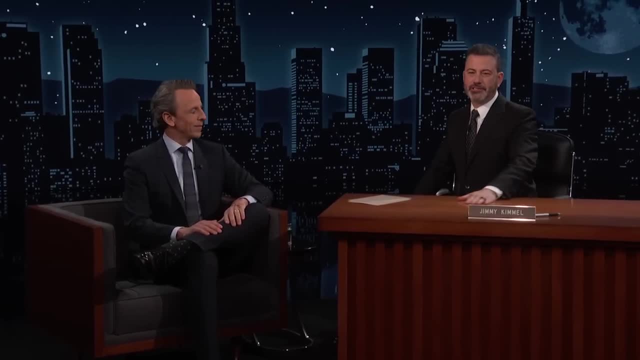 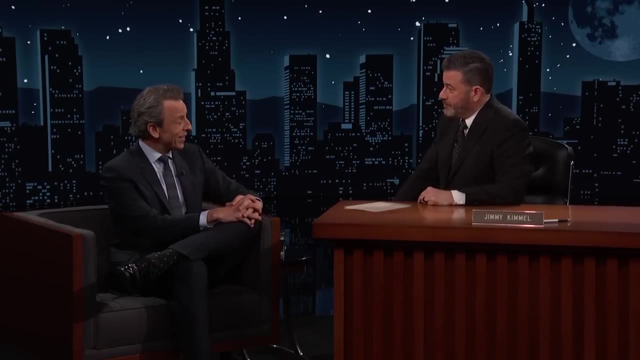 We'll be right back. We're back with the wonderful Seth Myers from Late Night with Seth Myers And also, you know, we hosted a podcast over the strike together. It was wonderful, It was a lot of fun, It really was. 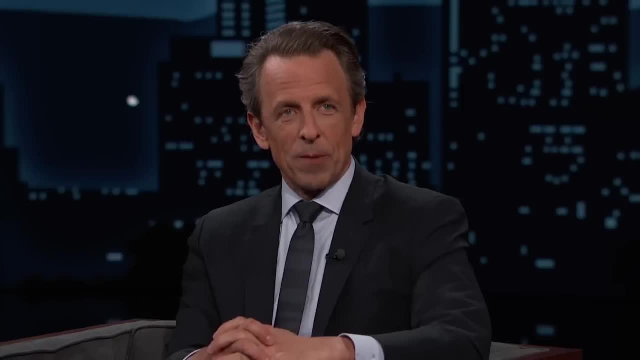 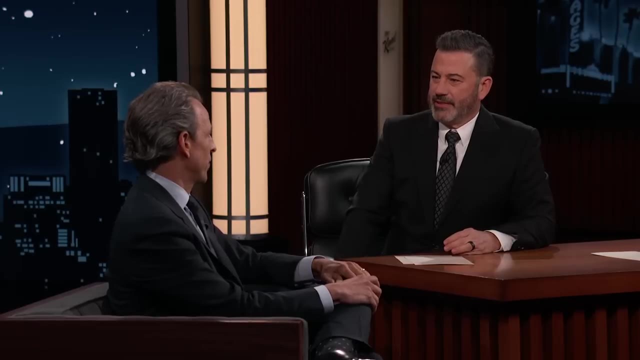 I think people are disappointed by how much fun we had together. I know I think people long for an era where we all hate each other and they're just bummed out that we found a common. Maybe we should give them what they want and start something, you know. 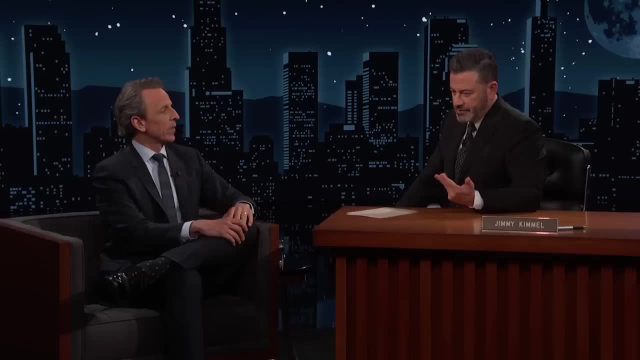 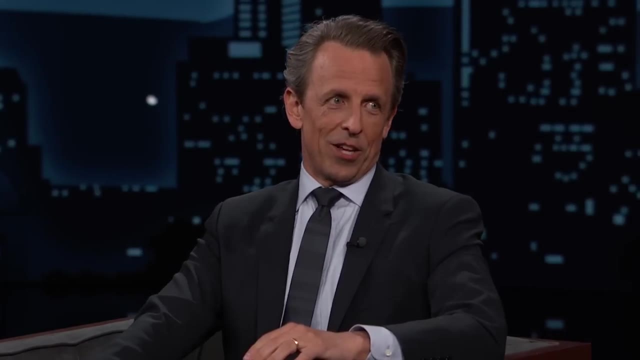 Okay, yeah, But it was you and me And John Oliver, Stephen Colbert and Jimmy Fallon. We did the show together. It was like an Avengers if they just got five lesser superheroes together and said: we want you to do a podcast about the Avengers. 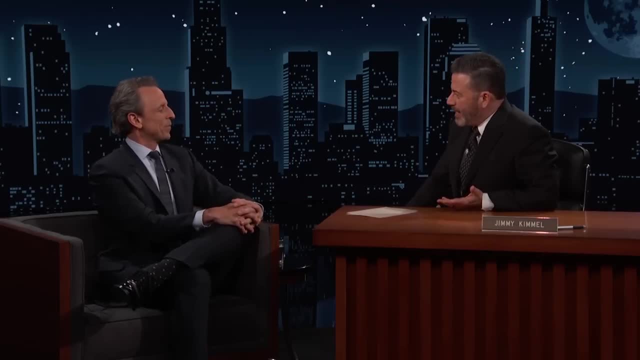 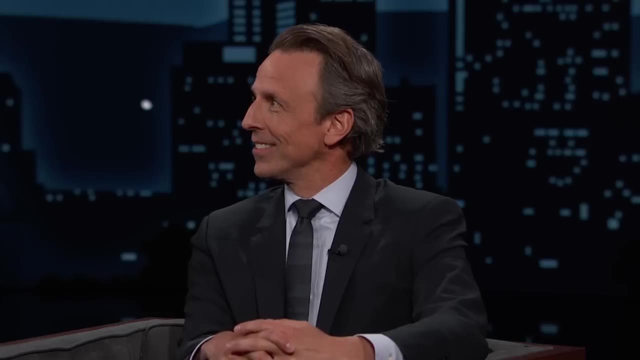 Like Hawkeye and his neighbors. Yeah, exactly. Do you remember the name of the podcast? Well, I think you're referring to Strike Force 5. It's a little. If you don't get it, you don't get it. 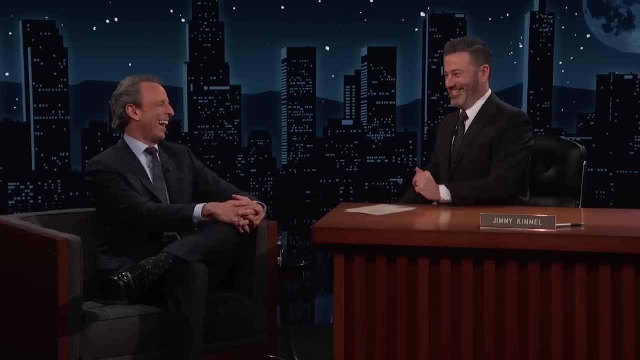 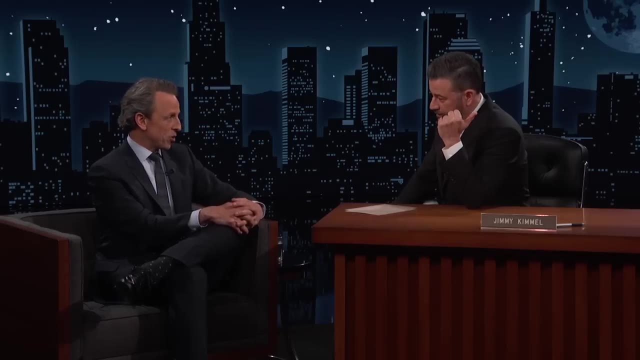 That's all. If you're not laughing, you didn't listen, Or they're not laughing because they did listen. Yeah, that's possible also. Yeah, You have a podcast with your brother, Josh. I do Family Trips. Which I was on was a lot of fun. It was a lot of fun to have you on It reminded me. I have to say I don't have a ton of memories of my childhood, but I remember every vacation. We only went on one vacation a year. 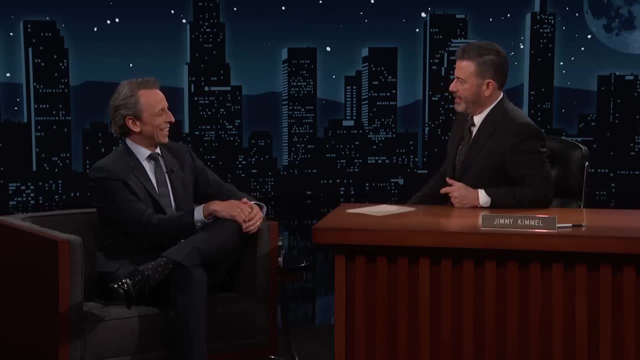 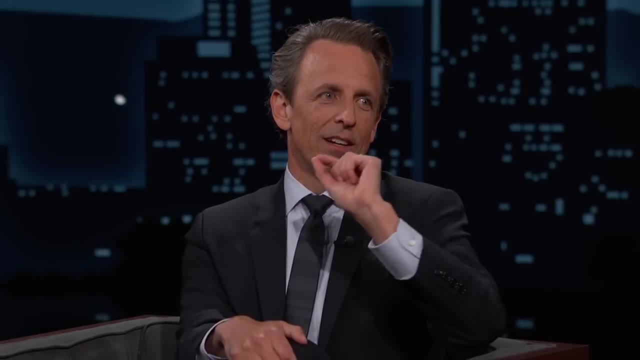 I remember every bit of every terrible vacation we had as a kid. That's sort of the thesis of the podcast. If you get people to talk about, If you get people to talk about their family trips, it turns out they have granular memory of details that happened. 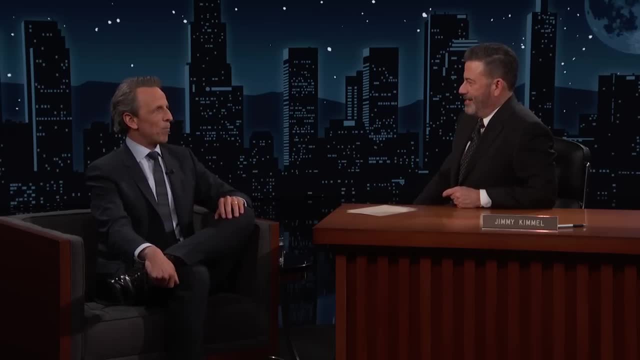 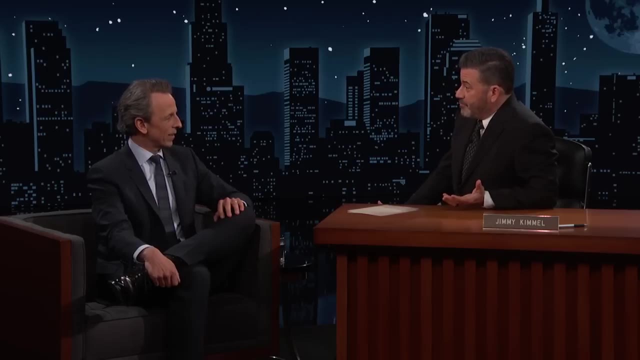 It's so specific, It's such a great idea. Yes, And I feel like people like knowing that everyone, for all walks of life, have had terrible vacations with their parents. Yeah, for me it turned out all of them were terrible, And when I was about 14, I just stopped going on them. 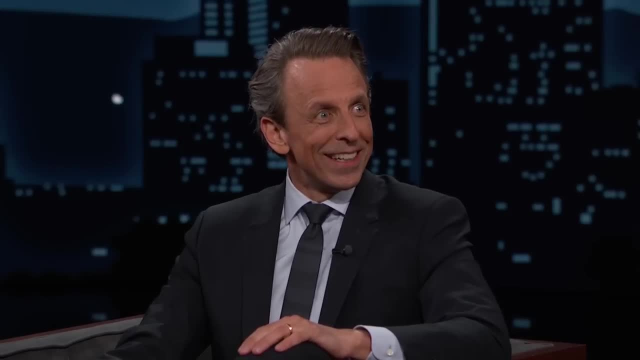 That's amazing. when you talk to people and you're like, wait, you're allowed to stop, You're not the only one who's like, and then I just said I'm not going anymore. and then I didn't go. It's a big reason of why I got a job at a young age. 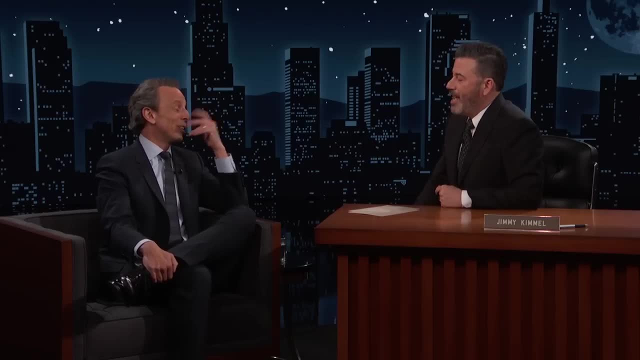 You're like I have to work this weekend. Sorry, Have fun. Yeah, well, it's effective. And now you have a brand new podcast that just started this week with the guys from Lonely Island. Yeah, so that's Andy Samberg, Kiva Schaffer, Jorma Ticone. 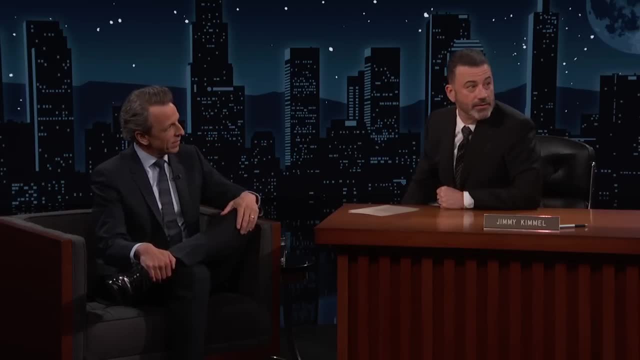 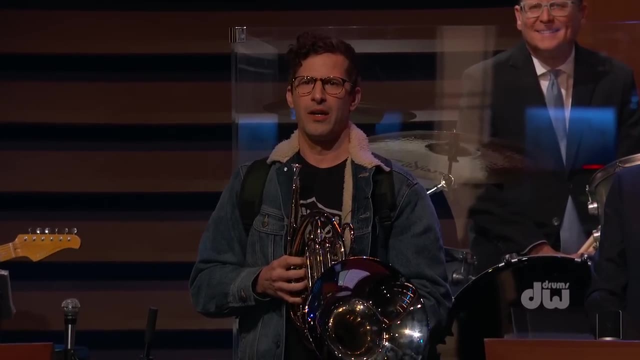 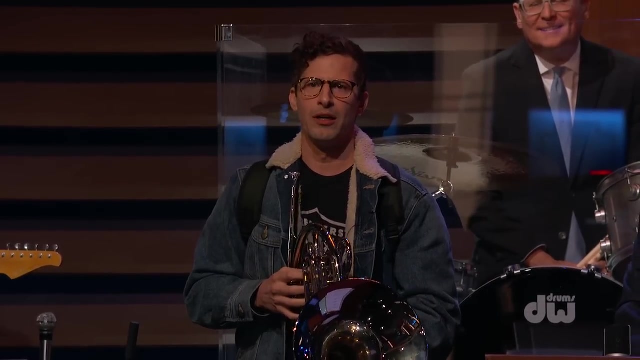 They did all the digital. Nobody cares What. I can't suck What is. Yeah, Literally everyone has a podcast now. I'm so sorry. I knew this was going to happen. I'm so sorry You knew this was going to happen. 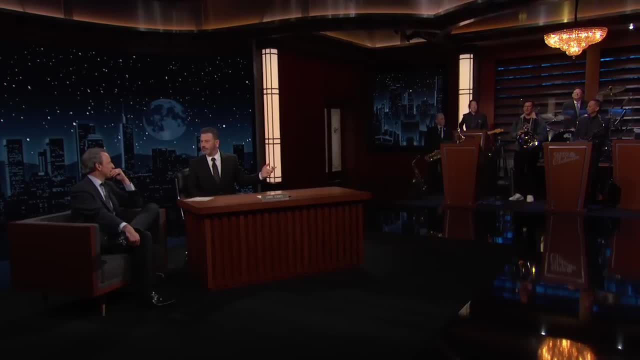 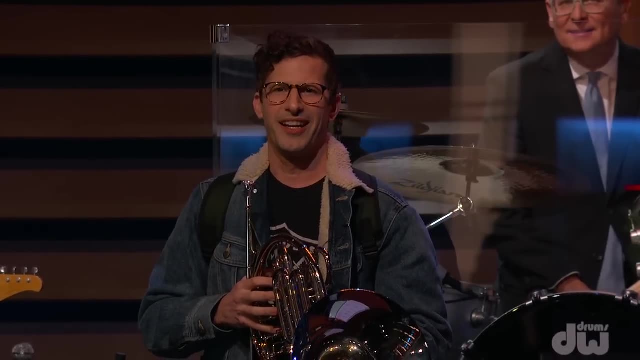 He really hates podcasts. Well, but he's on the podcast. How did you even get in here? Oh well, I was down the block at the wax museum, as I am every Monday, just you know, checking out my favorite waxies. 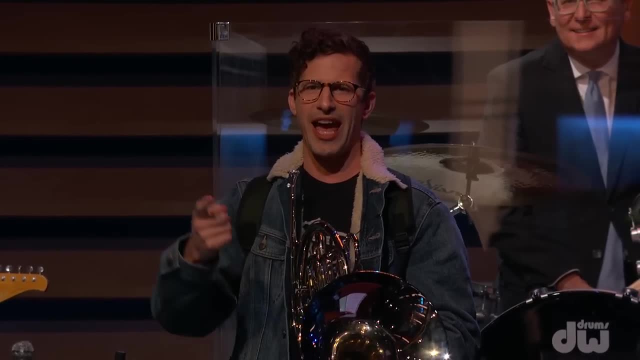 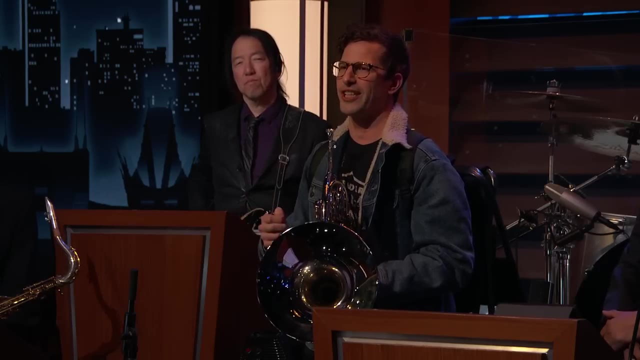 And I'm not sure if you know this, Jimmy, but you have one there, a figurine. Yeah, I do, Yeah, I do know that. Yeah, Yeah, Yeah. And do you know that if you pull down their trousers and 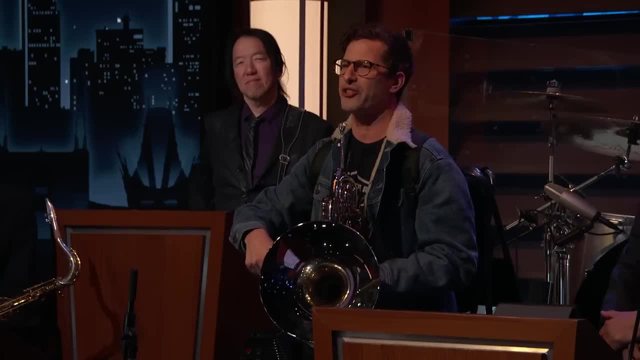 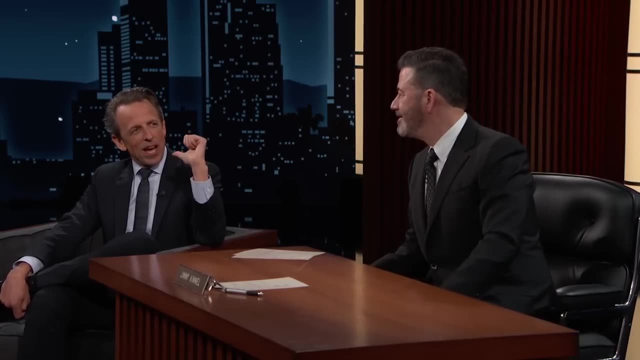 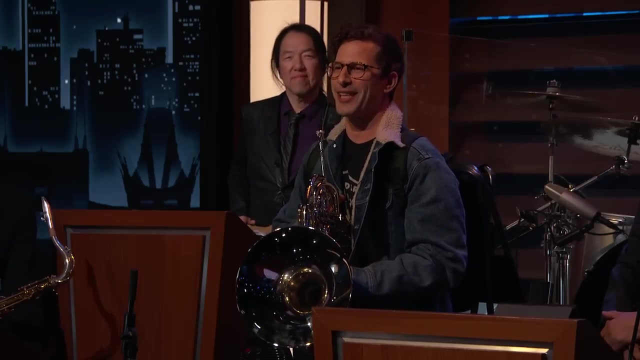 Climb into the butt. you go down a slide and it takes you to a tunnel that leads directly to your studio. Yeah, of course I designed. Yes, I designed that tunnel, Andy. do I have one? Yeah, but when you climb into your butt, you just come out of the mouth and it scares people. 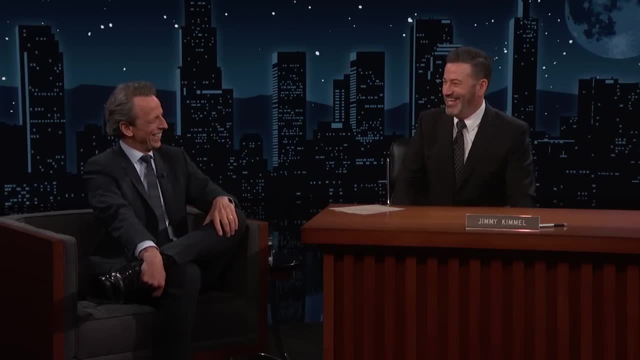 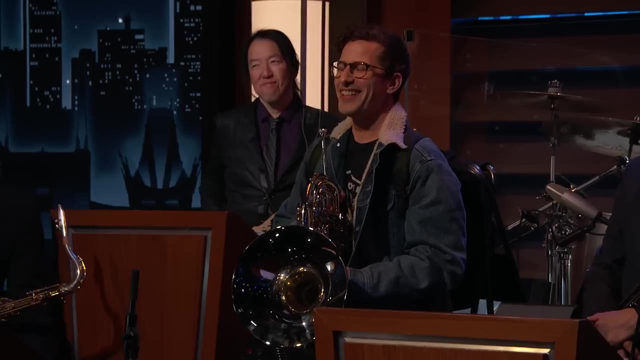 That's fabulous. That's not funny, That's terrible design. Oh well, we'll have to work on that one. I appreciate that design, Thanks. It looks like a billboard for American Horror Story. Andy-ways, that's how I say, anyways. 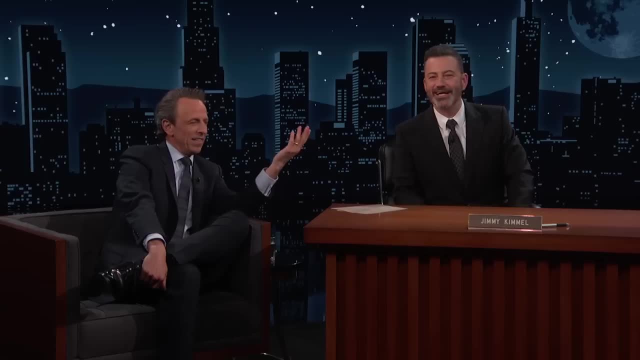 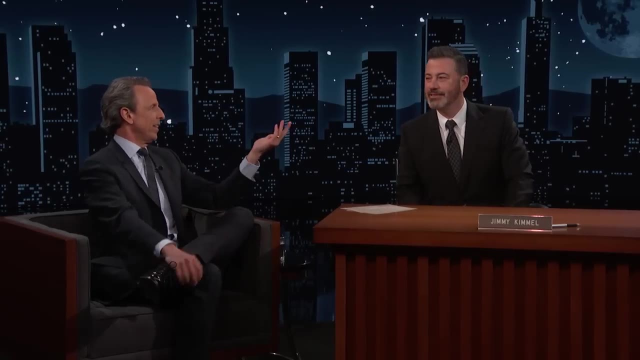 Back to the heckles Podcast. suck, Actually, Jimmy. the podcast I was going to talk about is the one that I co-hosted with Andy Samberg. Right, with Andy. It's about the work he did, the impressive work he did in his time at SNL. the digital shorts, which are iconic. 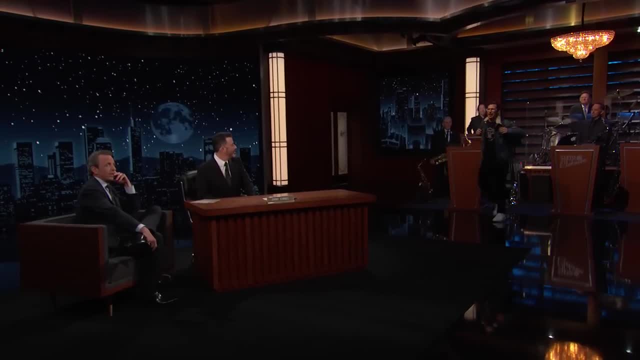 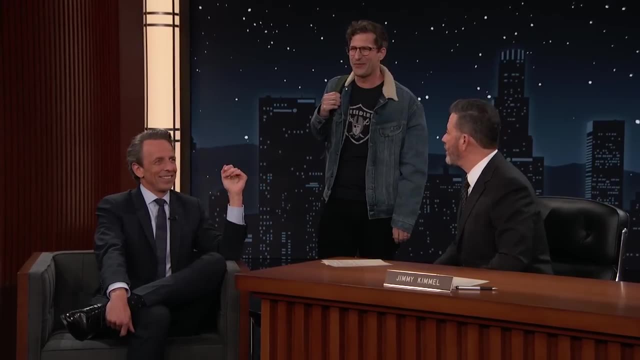 Right, yes, that's right, They were great. All right, I better get in there to make sure this thing's clear. Oh my God, Oh my God, Yeah, we don't Get in the work. Yeah, yeah. 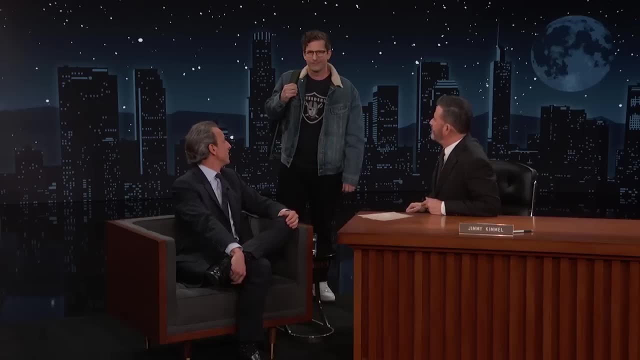 Yeah, we only have the one chair each, so you know we don't have a chair for you. Oh, it's okay, you guys, I brought my own. It's a backpack chair. Oh, So let me just. 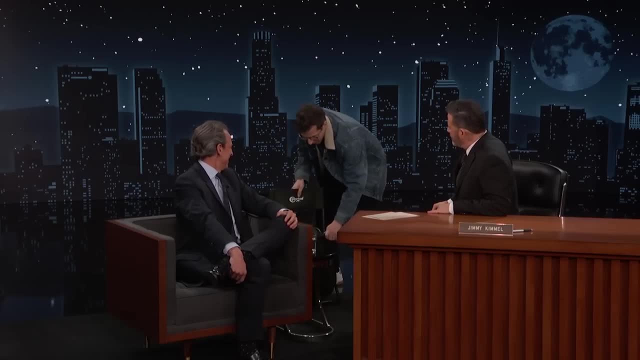 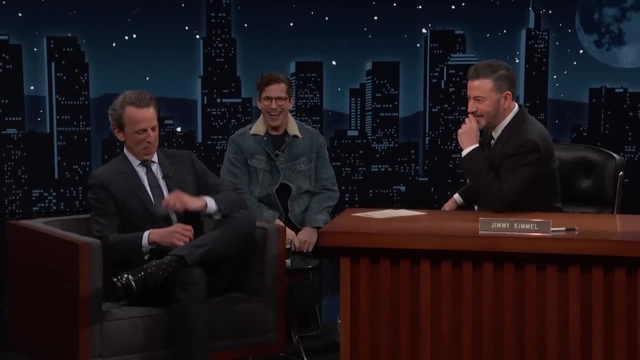 It's a chair. It's a chair that doubles as a backpack. There we go. Uh-huh, Yeah, I was just at Coachella, so it works pretty good. There's Coachella, So There we go. You touched on it. 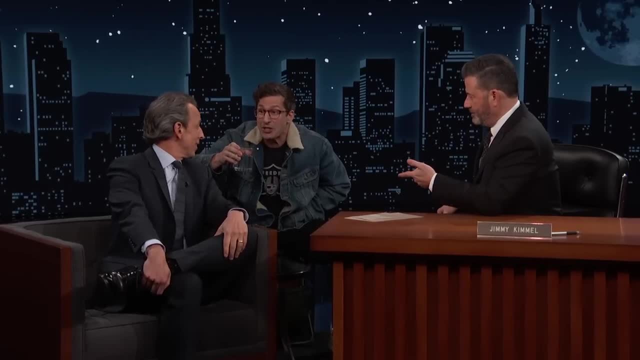 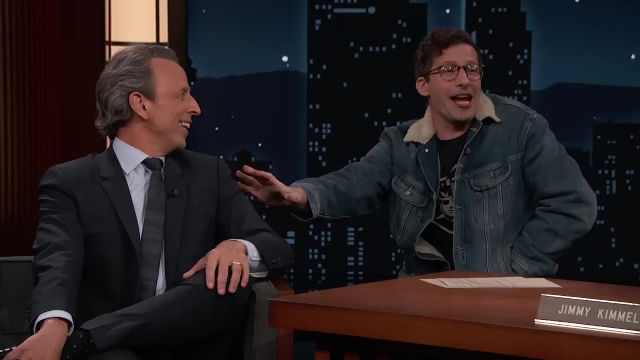 You touched on what the podcast is about. It's um. Can I have some of this? It's water. It's a little late to ask. You're supposed to ask before you start chugging it. We're old friends, Jimmy. 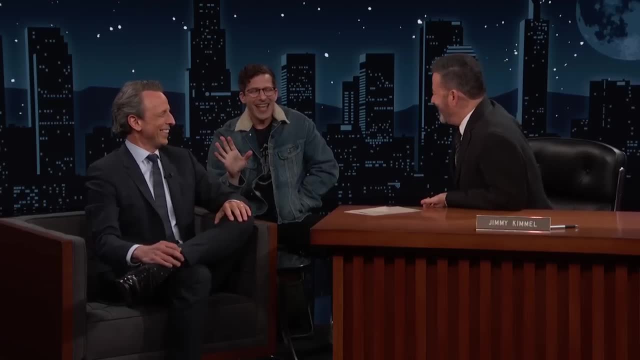 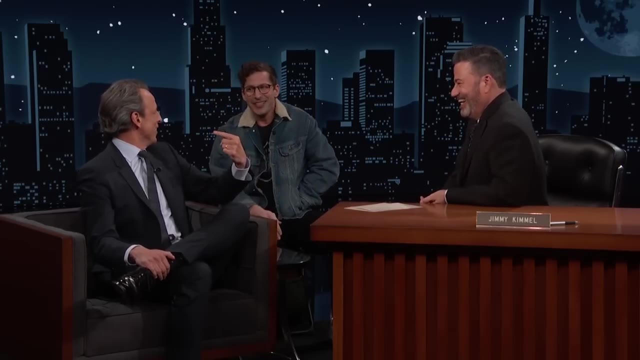 It's weird to see you guys together. I'm not gonna lie. Yeah, it's weird. Hey, be real. You guys talk about Trump. You couldn't hear us in the tunnel. Who knows Again, All right, sorry. 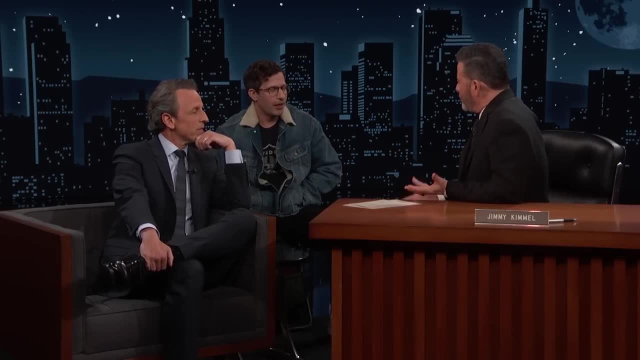 No, actually you're here. I might as well ask you- Yeah, I was gonna ask you about the podcast- What do you do specifically on the show? Oh man, it sucks so bad. Jimmy, You gotta check it out. 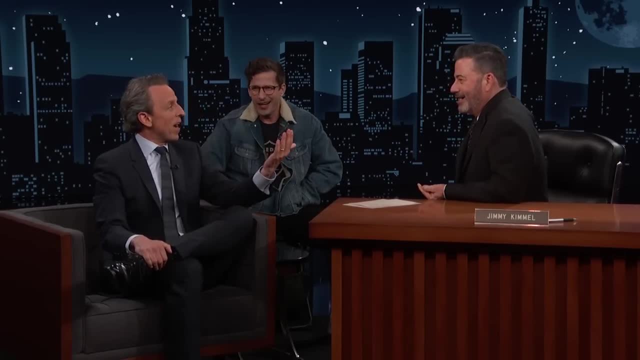 That doesn't seem like a great reason to listen to it. It is a great podcast. You know, and again, you know, Andy, I'll be honest, he doesn't like the art form of podcasts, Is that right? But he's very good on the podcast. 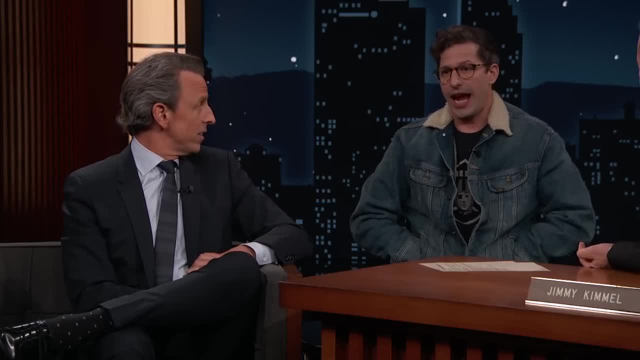 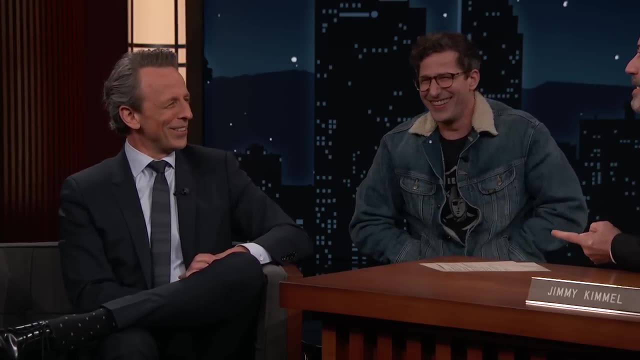 and we talk about the very fun times we had together at SNL. Yep dragged, kicking and screaming. I was told there's gonna be a massive payout. Is that what they said? How many Lonely Island shorts are there? There were 110, we think Lonely Island shorts. 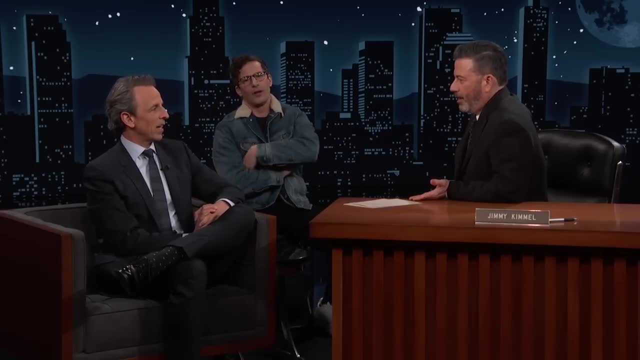 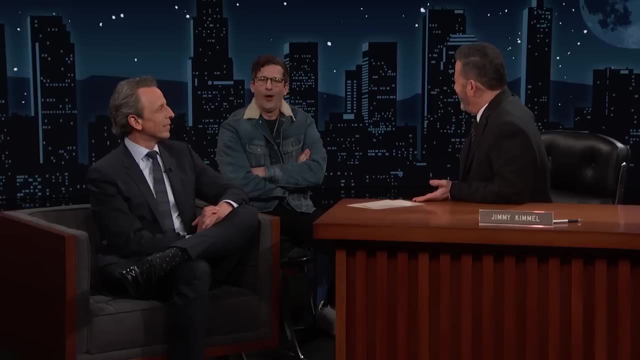 So then this would be capped, this series at 110 podcasts. I would be shocked if, based on Andy's behavior, we make it to 30.. No, that's fair. You think you're gonna make it past 30?? 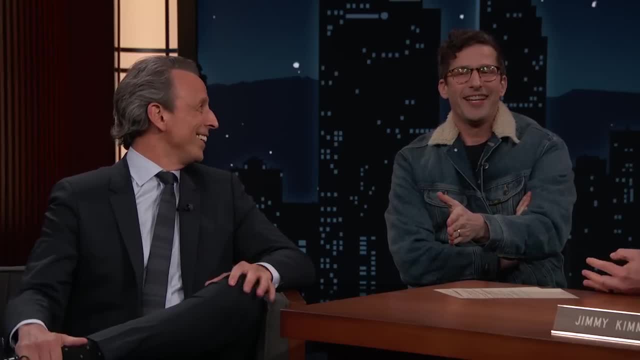 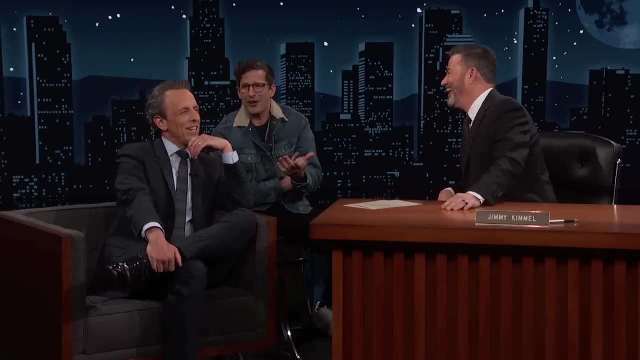 No, We're gonna go the whole way Uh-huh. And here's the thing about podcasts. Okay, great, Even though they suck. ours is great. You gotta check it out. Nice, Can I? How You guys. 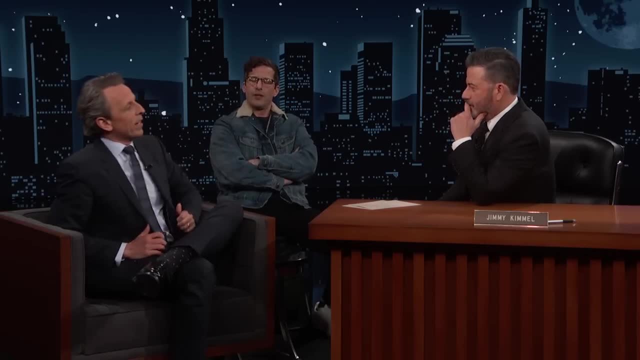 Did you meet on SNL or did you know each other before We met on SNL? and one of my favorite things about Andy, who I love very much and I think is a genius- did not like him right away. Oh really. 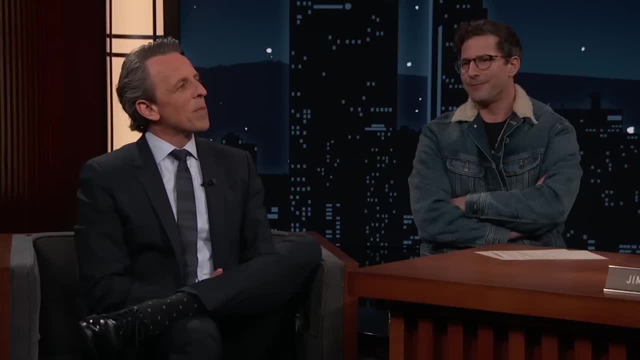 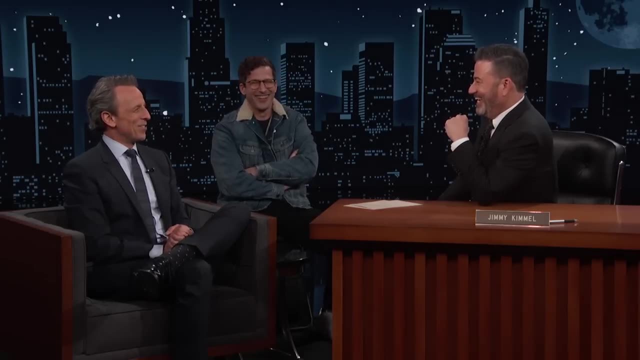 I thought he was a good dude, but I thought his comedy was very sophomoric. Right, Okay, Now you know better. Yeah, now I know better. Now he plays the French horn. Yeah, exactly Now he does comedy about crawling in butts. 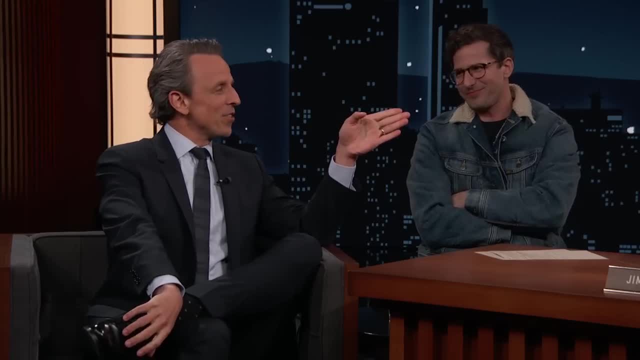 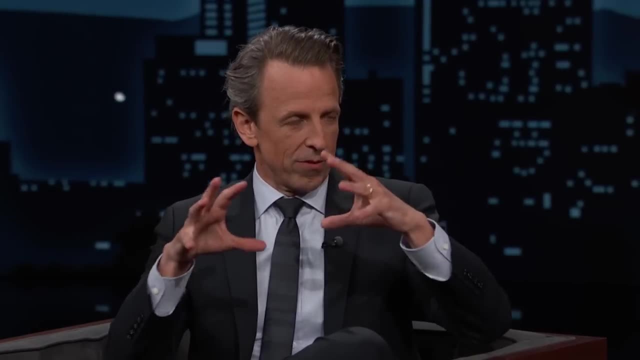 Wax butts, but go on. So Andy used to do this bit. We would write very late at SNL on Tuesday nights and I'd be at my computer and he would come into my room and I'd be the stress of trying to write a sketch.